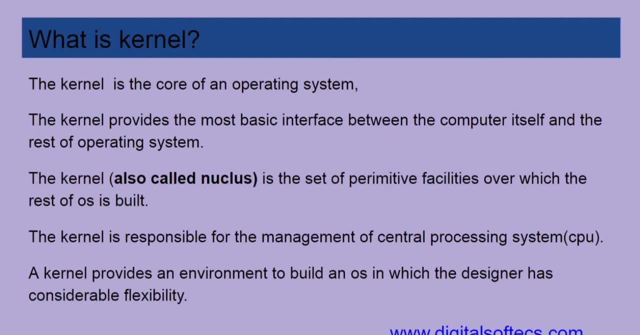 important to the software and hardware. and the operating system resides on the kernel itself. So half of its kernel provide functionality, half of it is reserved by the operating system. So kernel is the core of an operating system. You can say kernel is an operating system, but the kernel provide the basic functionality. 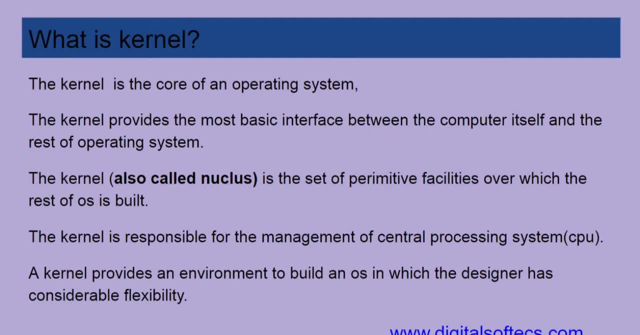 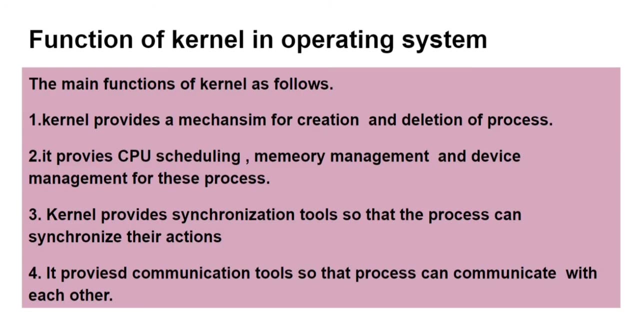 and manage the different resources of computer hardware. So the kernel is responsible for the management of CPU central processing unit where we have management of processes. So what are the different functions of kernel? So after the functionality of a kernel you will be able to see what are the responsibilities. 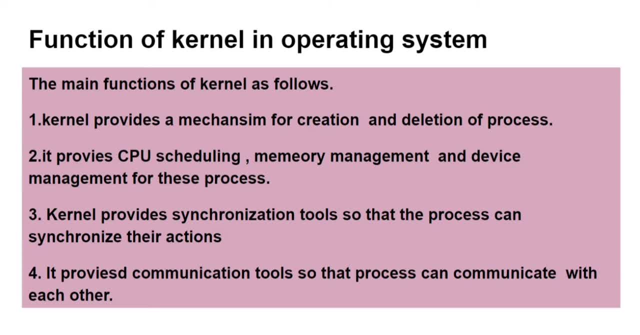 of a kernel. So the main functions of kernel are as follows. Number one, kernel, provide a mechanism for creation and deletion of a process. So process is one of the most important part of operating system And there is a managed operation. 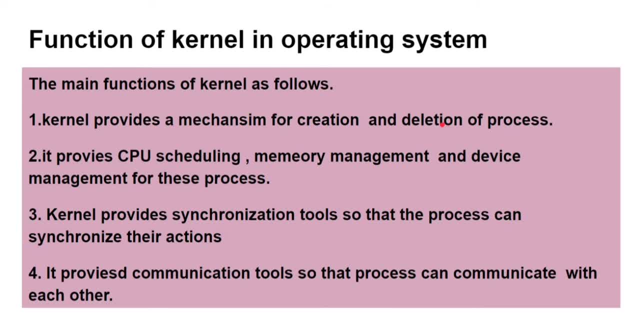 And by the operating system. we call them process management. So kernel provides a mechanism that how we can create process and how we can delete process. So it is a very basic process of computer system or function of a computer system. Number second is it provides CPU scheduling, memory management and device management. 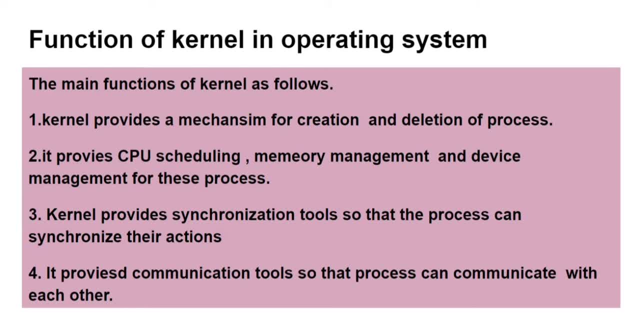 for these processes. So kernel deal with the creation of process and deletion of process And it manages. So kernel manage CPU scheduling, It manage that which process will executed, which process will wait and which process will end. So they provide memory to that process. 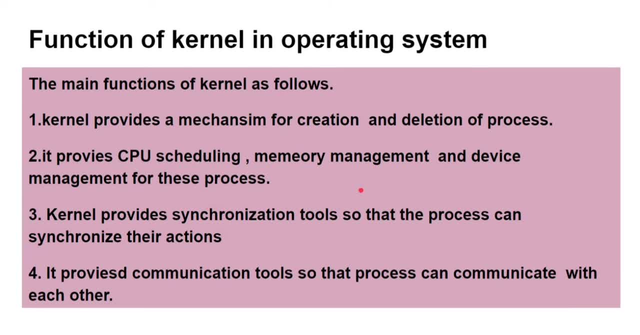 And device management for these process, such as input devices- So which process use a keyboard, which process use the speaker, and everything that is input, output devices and other devices or device drivers. So it is managed by the kernel, So kernel manage CPU scheduling. 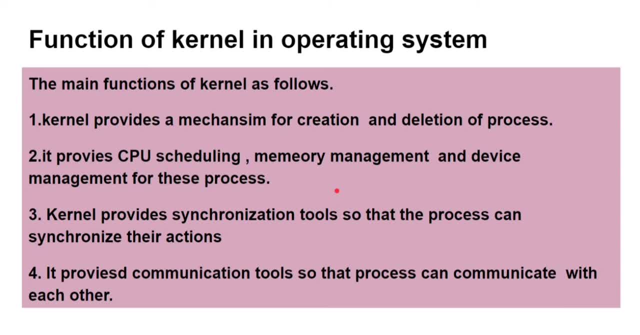 And memory management and device management. the devices which are connected to the computer system- So number three is kernel- provides synchronization tool to that process- can synchronize their actions. Synchronization mean something happens simultaneously. So we can see that during a process, between process one and process two there is a very 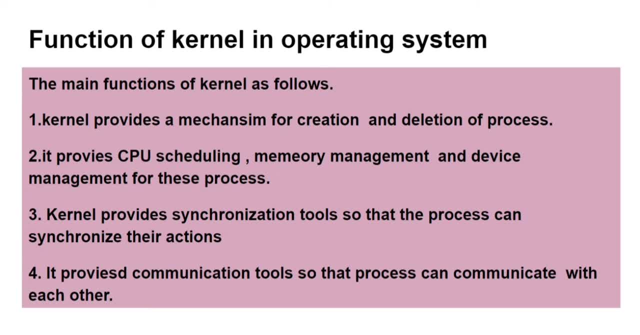 little space. So kernel manage this spaces, As you see earlier I said, between process two and process three. so what happens where all the components will be synchronized, alter it. So here, by using the kernel manage process tool, we get easy. 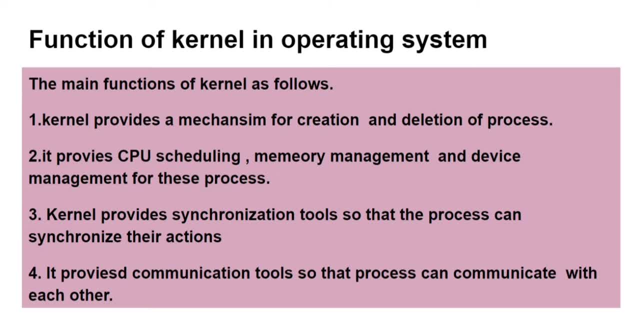 permission for us. Let me explain today. So first of all, Hola, Quick, kaboom back. process ads among the executioner process, such as playing a video and printing a document, is a two process. so kernel manage these two which are different process, and kernel manage itself. 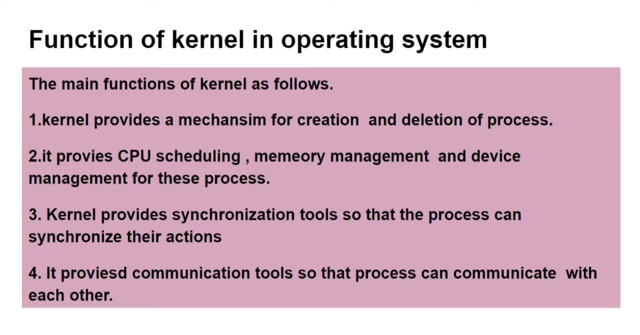 the process: printing of device, printing of papers and playing a video. so these are different process, but kernel manage these things with the help of management, with the help of process management, and a process have a lot of actions, such as printing a document, changing in the document. so are these actions were managed by the kernel. so number four, one, it. it provide communication. 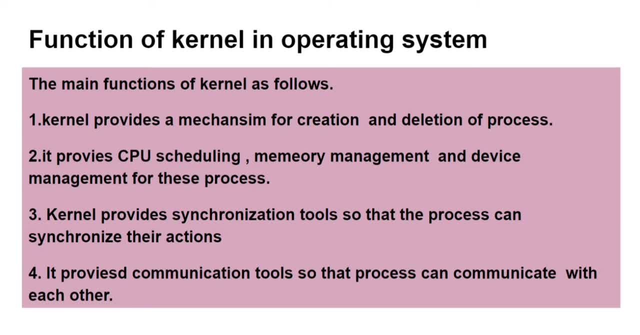 tools. so, though, so that process can communicate with each other- very important, like if we have command in action in during the processes, so different processes can communicate with each other, like printing a document and editing a document is a very a small process, but kernel manage these things, and kernel manage a word, document playing, a videos, everything that actions are managed, so 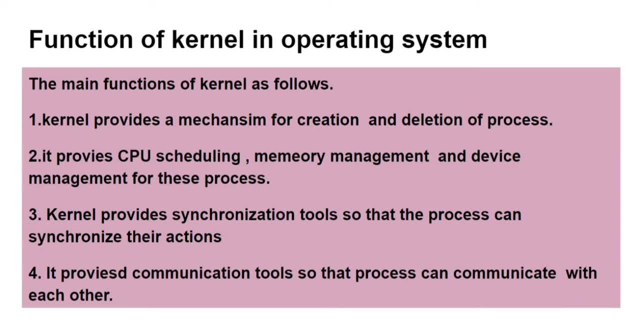 when we have a communication among processes, so kernel managing. so these are the main functionality of a kernel: kernel provide mechanism for creation, deletion of process, CPU scheduling, memory management, device management. kernel provide signalization tool to the process and it provide communication among the different process. so when the processes are communicating, so they will execute in a special 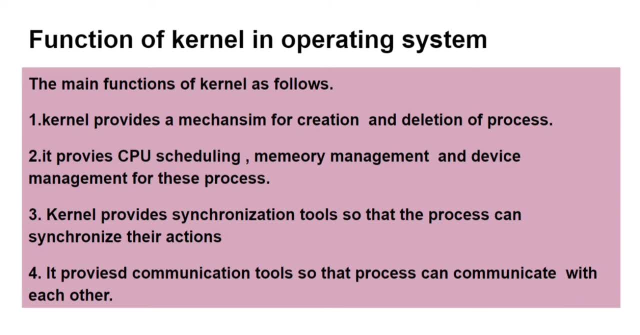 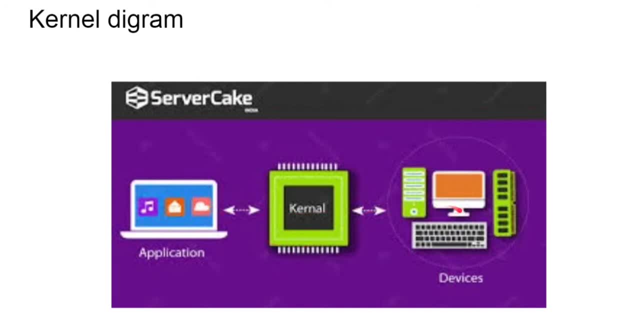 sequence. so these is the very important function of kernel. hope you understand this things. so this is the kernel diagram. so we have applications, we have kernel and we have devices. so it is a bridge among the software and among the hardware. so kernel manage devices and kernel manage itself'. 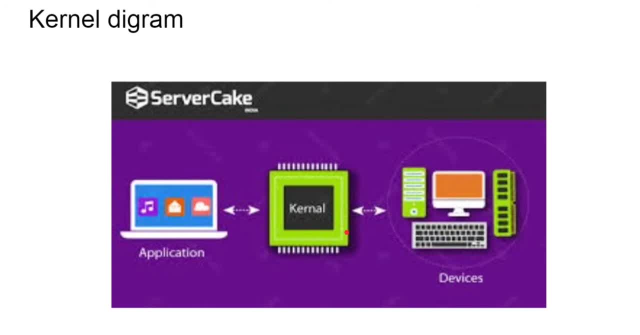 1961 on the device of 40 content deploy full realistic generation of products. has a, b sending operators. computer memory chip declaring test is the forth in the query of the hardware, dex code operating system and the management of different things such as process management memory. 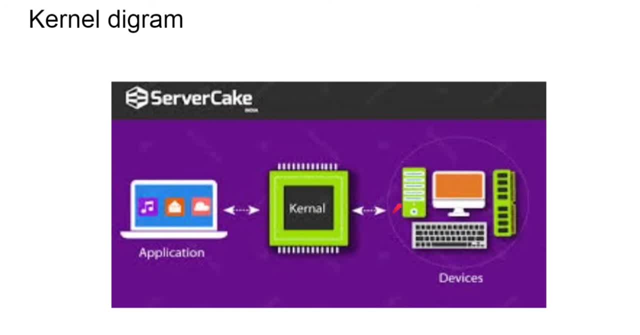 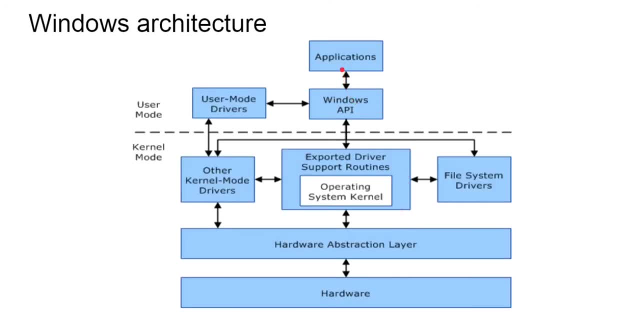 management and processes, communication. So all these things are managed by the kernel. So we have the Windows architecture. You can see, we have the application. we have Windows API user-mode drivers, so there's other kernel-mode drivers. So this is the kernel-mode. 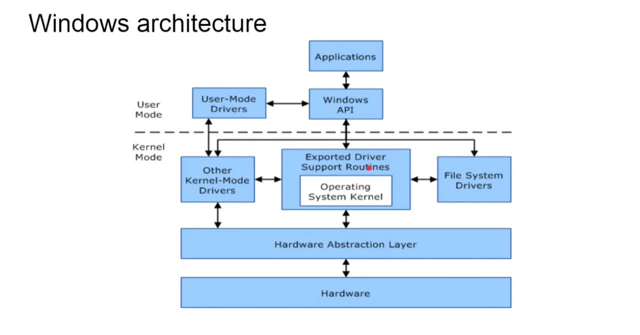 So kernel contains a lot of things. It contains the exported driver support routines and they have operating system kernel. So look at that. Kernel is here. Kernel is the core of operating system. We have file system, we have hardware, we have hardware abstraction layer and we have 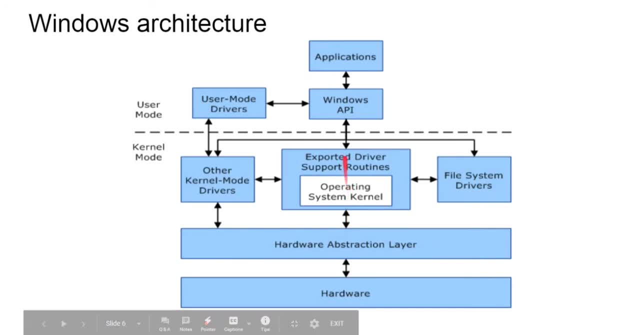 a hardware. So kernel is a bridge among the applications and among the drivers- Hardwares. So these are the functions and these are the main area where the kernel is. So it is the nucleus of operating system. It is a simple picture of Windows architecture. 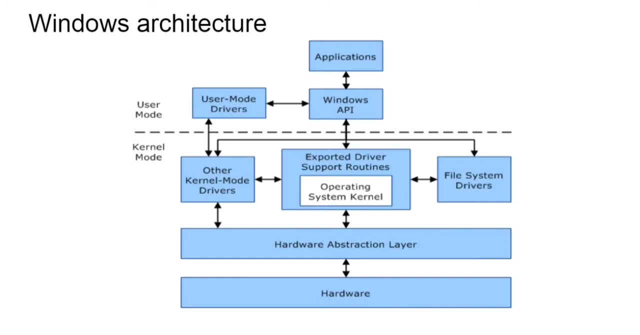 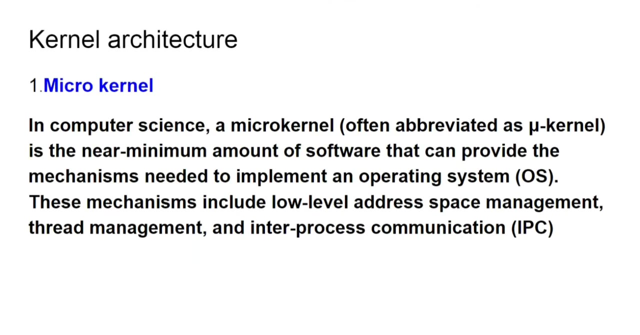 You can see different kinds of functionality applications, Windows APIs and exported driver support routines. We have a hardware abstraction layer and hardware. So these pictures are taken to just a clear view of where the kernel is reside in operating system. So we have a kernel architecture. 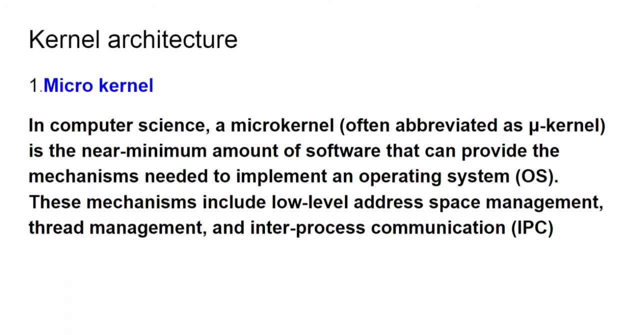 We have number one microkernels in computer science and microkernels are often called abbreviated as a Sigma. kernel is the near minimum amount of software that can provide the mechanism need to implement an operating system. So implementation of operating system is done by the kernel. 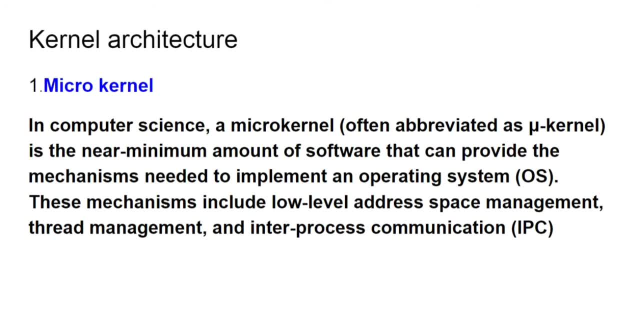 So there is the microkernel. Microkernel is one of the most important part of kernel, So these mechanism include low level address, space management, thread management and inter process management, called an IPC. So in computer science we can see that the minimum amount of software 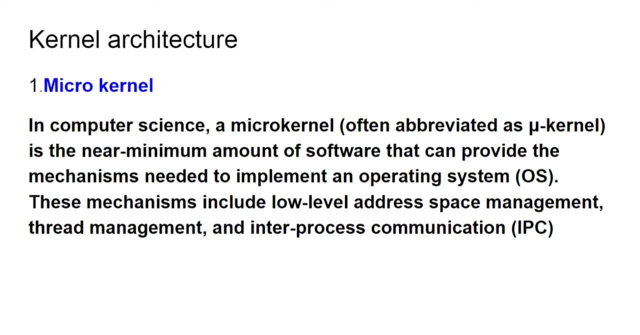 That provide the mechanism need to implement operating system. So implementation of operating system is done by the kernel and that is important part of kernel card microkernel And they have mechanism such as memory address, space management, thread management. So these are the important functionality provided by the microkernel to implement the operating. 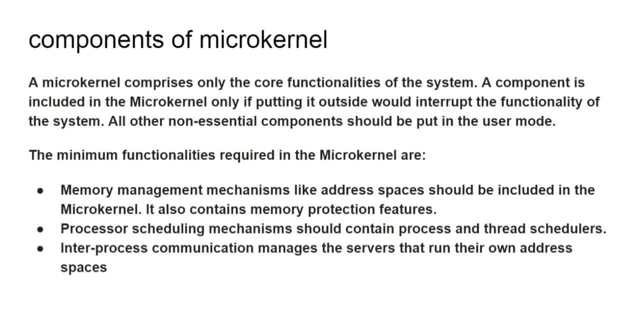 system on the hardware. So components of microkernel. So a microkernel compresses only the core functionality of system. A component is included in the microkernel only if putting it outside will interrupt with the functionality of other system. of the systems. all other essential components should put in a user mode. so 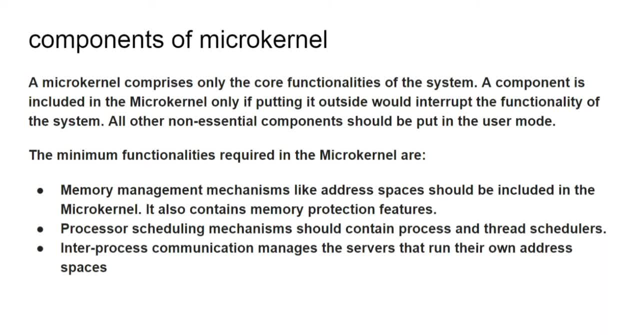 let's see the functionalities. memory management mechanism, like address spaces, should be included in the micro kernel. it also contain memory protection features. process scheduling mechanism should contain process and thread schedulers and enter process IPC communication manage the server that run on their address spaces. so these are the very important functionality of 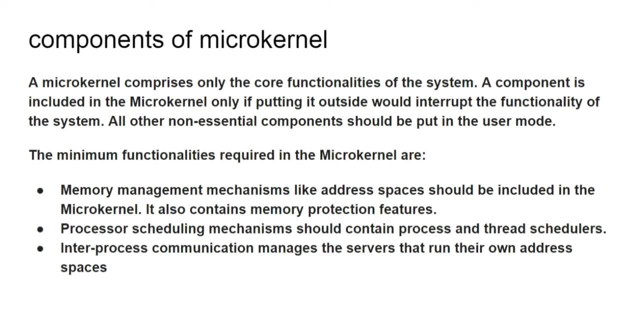 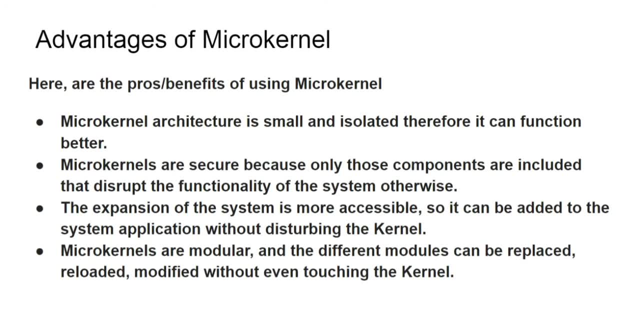 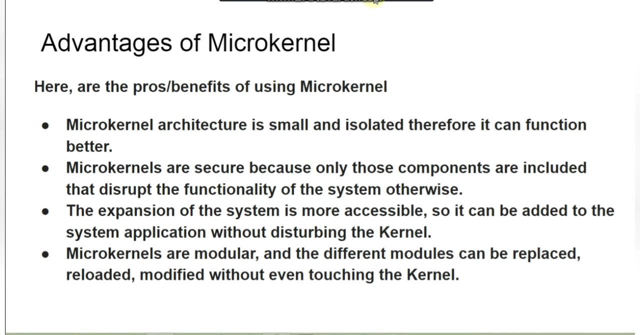 microkernel and is the. this is the component of a microkernel and you can see the functionality of microkernel. so if we have the advantages of microkernel, so advantages of microkernel. here are the pros and benefits of using microkernel in microkernel, architecture is small and isolated, therefore it can. 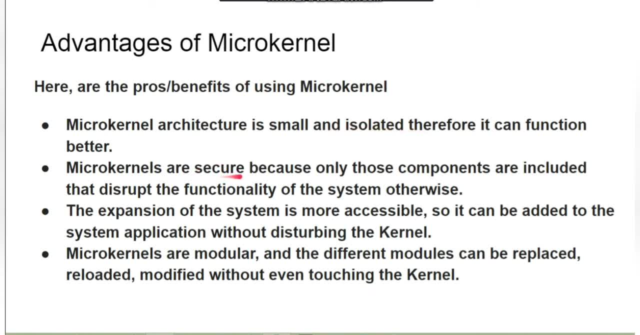 function better. Microkernels are the secure because only those components are included that disrupt the functionality of the system otherwise. So the expansion of the system is more accessible, So it can be added to the system application without disturbing the kernel. So microkernels are modular and the different modules can replace reload. 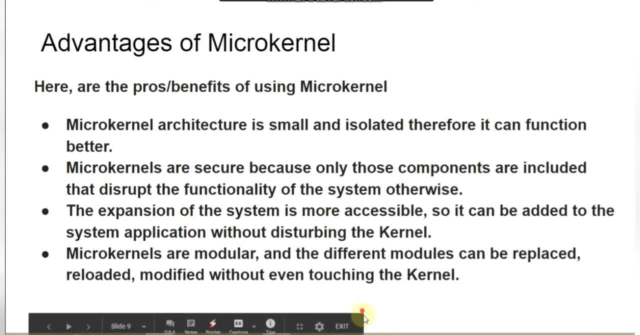 modify without even touching the kernel. So the benefits of kernel is that that architecture is small and it is isolated, So it does not disrupt the operating system or the other important part of kernel where the operating system is reside. So microkernels are secure. 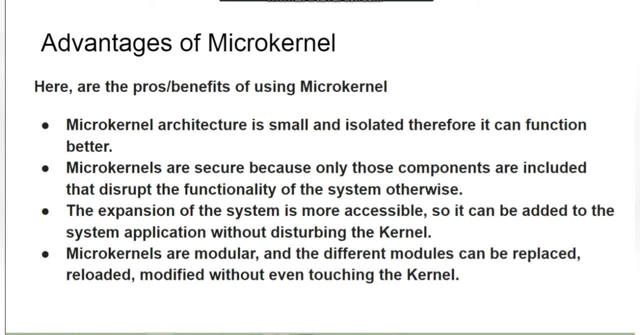 because only those components are included that disrupt the functionality. So the expansion of a system is more accessible. So expanding the system is very basic. So expansion is done by the microkernel. So due to the microkernel advantage we can expand our system without 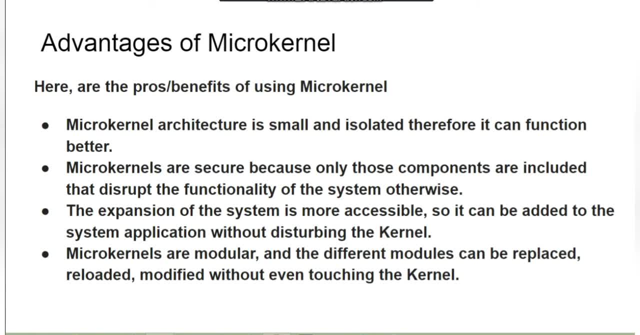 disturbing the kernel. So microkernel, modular or a different modules can be replaced: reload, interrupt without disturbing or touching the kernel. So this is the functionality of microkernel: to code it, not a disrupt the kernel and expand their functionality, accessibility and a different. 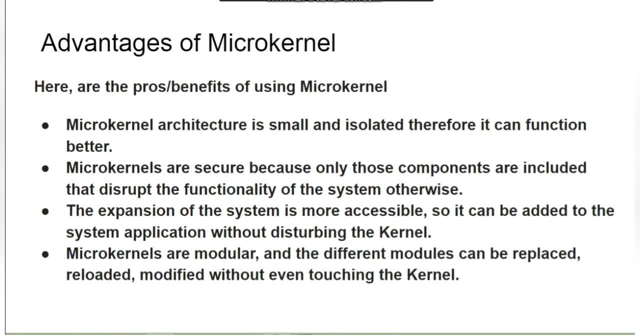 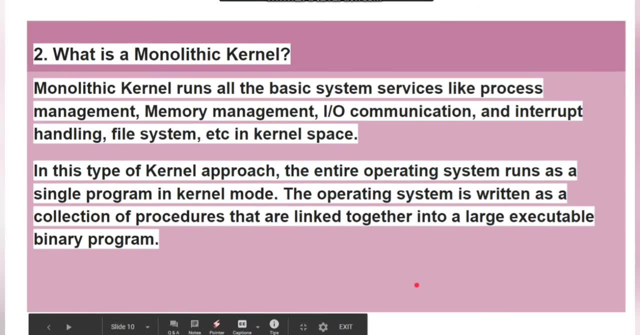 module replace replacement. So these are the functions of microkernel. So we have a what is monolith, Monolithic kernel? Monolithic kernel runs all the basic system services like process management, memory management, IO communication and interrupt handling, file system, EDG and. 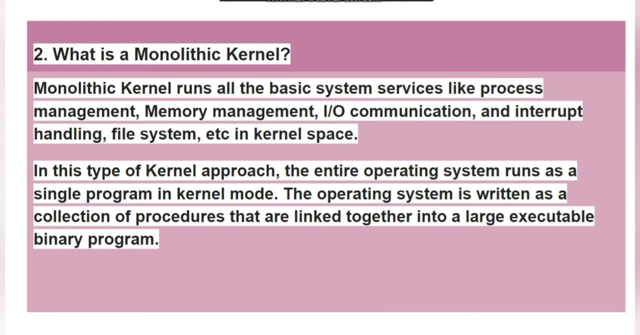 kernel space. So microkernel works as the resization of operating system, such as the accessibility expansion and everything that is Now the different management is done by the monolithic kernel. So monolithic kernel runs the basic system. So the monolithic kernel runs the basic system. 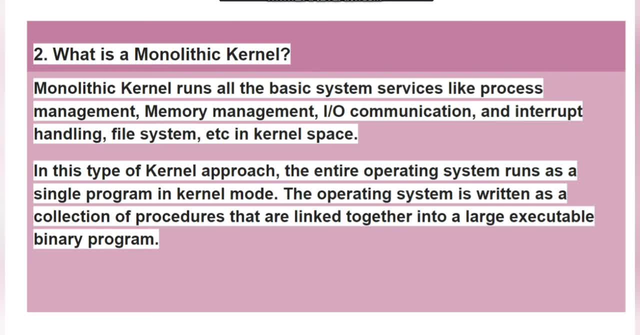 like the process management, memory management, IO communication and interrupt handling file system. So the part of a kernel which manage these processes and memories are the monolithic kernel. So monolithic kernel manage memory management, input, output, communication and interrupt handling file system. So all these things are included in operating system, which 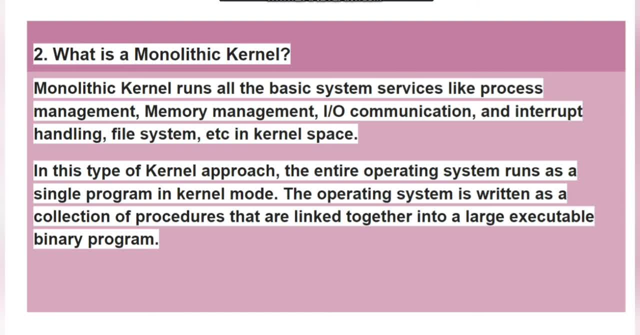 is controlled by the monolithic kernel And this type of kernel approach the entire operating system run as a single program. in kernel mode The operating system is written as a collection of procedures that are linked together into a large executable binary program. So very important concept here. we have points here. So in this type of kernel approach, 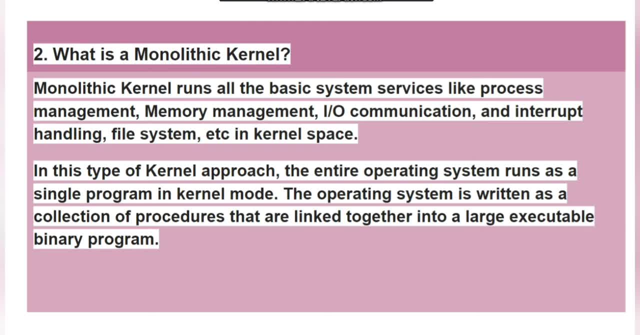 the entire system is run as a single program, like an in kernel mode. So operating system is written as a collection of procedures. Now the operator. what is an operating system system? Now, as we move on forward, we can understand the basic definition of a operating system. Here we have the operating system is written as a. 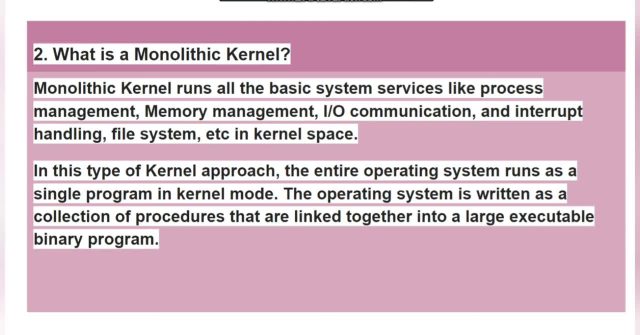 collection of procedures. So you can say, when somebody asks you what is an operating system, you can say that the operating system is written as the collection of procedures that are linked together into a large executable binary program. So these are the thing the monolithic kernel manage, the basic. 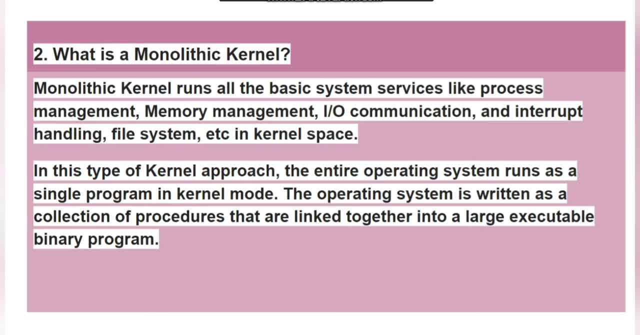 processes and the basic functionality of operating system and management is the responsibility of kernel and there is monolithic kernel, the important part of our kernel. So memory, management and communication interrupt. everything is managed by the kernel. So it is all about the kernel We have.